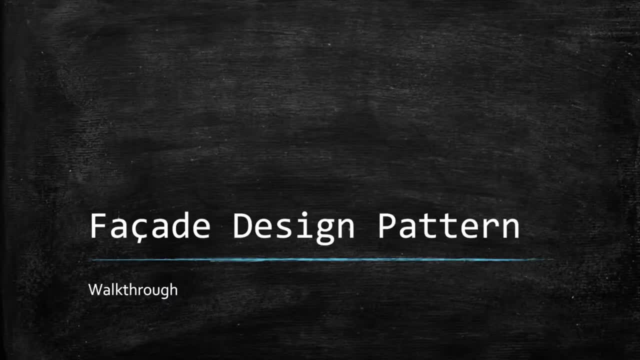 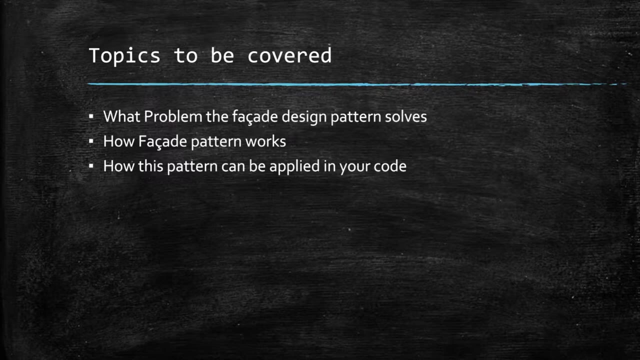 Hello, all welcome to the design pattern series. Today we are going to look into facade design pattern and we will go through all the details and how to implement it. So let's start. Let's go through the theory part first and then we will look into example to understand how it works and 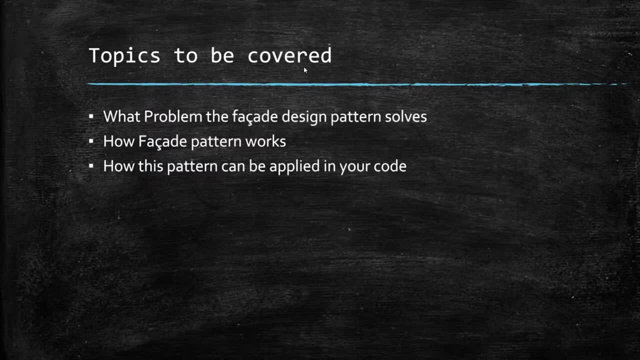 how to implement it. So in today's video, actually, the topics which we are going to cover are what problems the facade design pattern solves, how facade design pattern works and how this pattern can be applied in your code. So we will look into all the aspects of this particular design pattern. 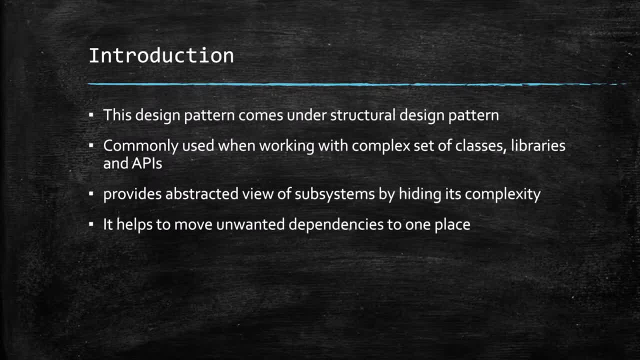 Okay, now moving to the introduction part. the facade design pattern comes under structural design pattern, and facade design pattern actually is useful when you want to handle complex systems which has multiple independent subsystems. Like example, it will be multiple classes or modules to achieve the desired functionality. So you want to do something you will need to call multiple. 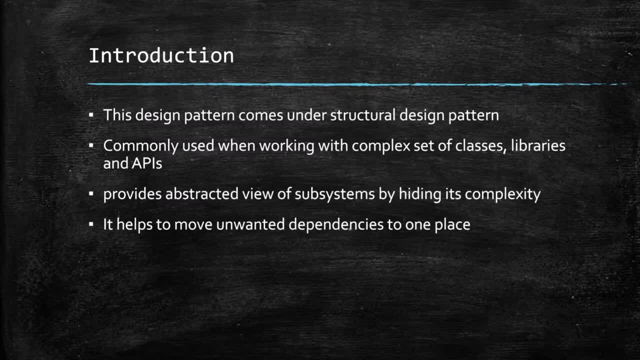 classes and subsystems To perform that particular task and to handle such a situation. this pattern actually works, and this pattern- how this pattern works- is by providing a simple interface for subsystems which are poorly designed or complicated, and it does it by hiding the implementation details. In other words, it provides 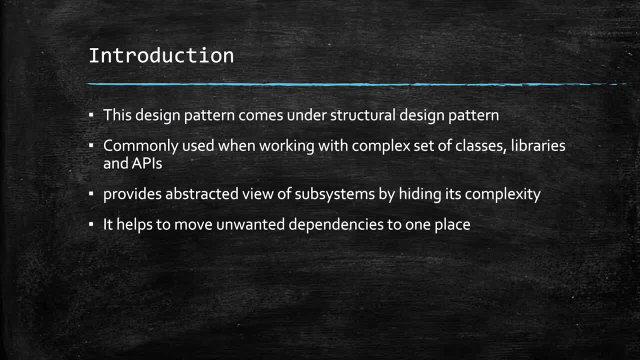 abstracted view of subsystems, by hiding its complexity, which result in offloading all the load from client classes or the system. and, as of now, this might not give you a complete picture about facade design. So let's go ahead and start. So let's go ahead and start. So let's go ahead and 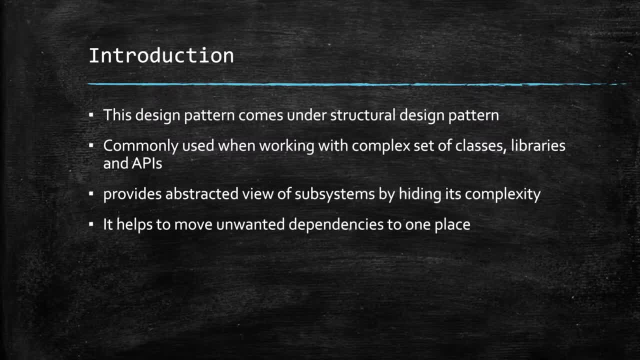 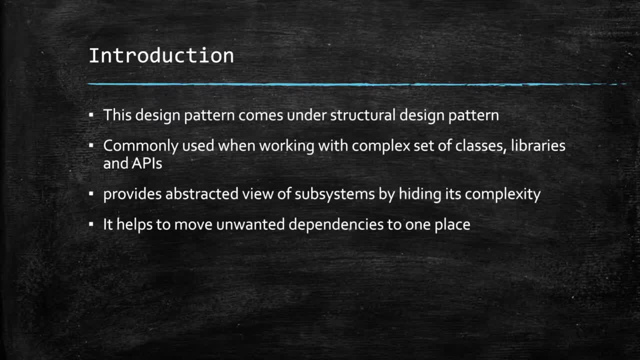 happened, two that hardly ever happened to him at all. In that case, will find once we actually really analyse how he acid tässä purpose of the construction: calculate the solutions said to utilize a certain type respond throws and which will result in, by end of the day, like class being tightly coupled with the multiple. 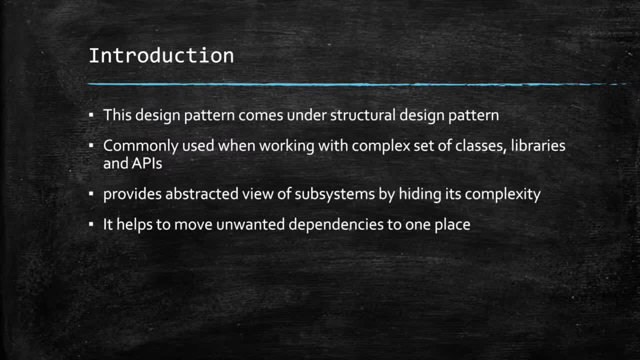 classes. simple example to be given will be uh like if a client class wants to save data in database and if you have uh exposed, separate method for each step. uh example will be like one method for validation, the other one for logging into data, other one for adding the data and so on. so there 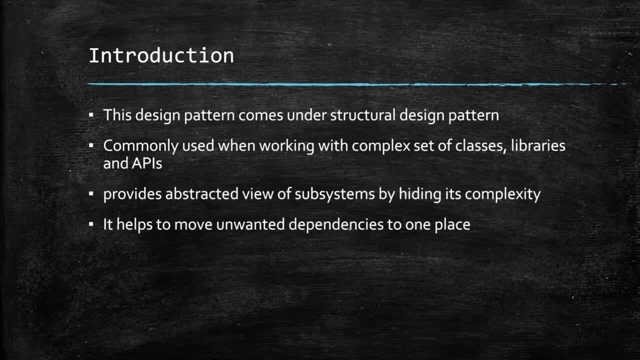 might be multiple uh checks you want to perform, or you have, or or few couple of methods. so in this case, in case if you uh all these meters actually you provide to client or to consume, and then client will do this, will need to decide like which method to call and at which point. because in case 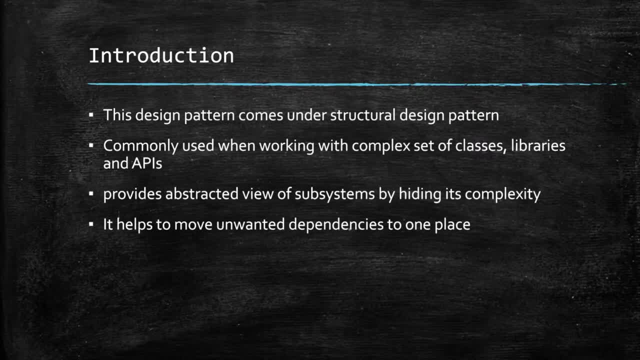 if it fails to call the validation method and, while saving the data, we don't have proper uh like check to see if the data is correct or not, or whether we must store it in database or not. so in that case, wrong data might be used to save the data. so in that case, it might be used to save the data. 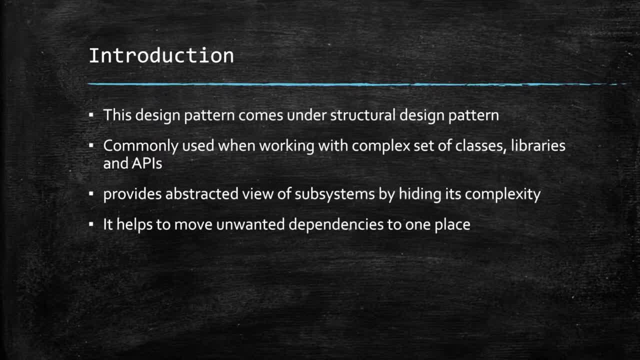 might go to the database, so this kind of things might happen. so, to come with the situations, what we can do is we can provide a class which will take care of all the steps and provide only one method, like add data, which will take care of calling all the steps. so this particular class. 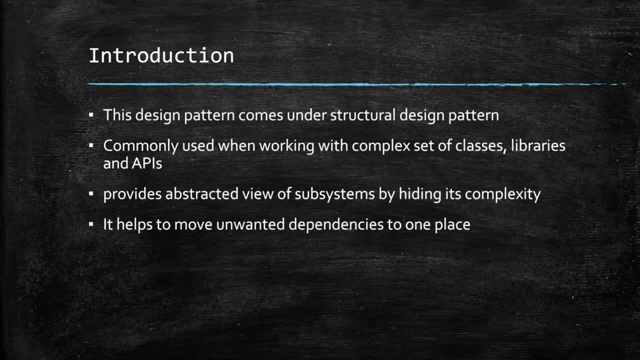 what it will do. it will call all the intermediate steps in a particular order, so client don't have to bother about calling them what client will do. like. client will call this new facade class and using that one method only it can perform all the operations and this will also remove the tight coupling from the client. 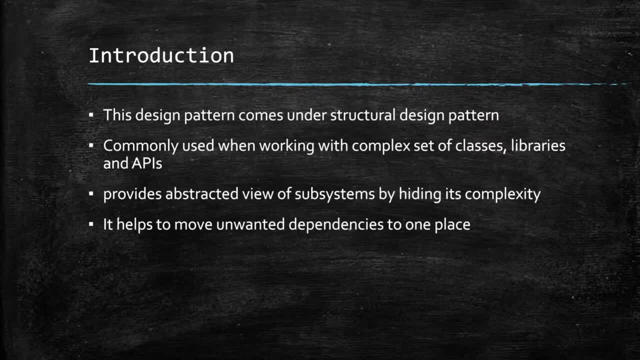 classes. by this way, actually, we are making sure that client class is calling only one method and not the complex system directly, and even if in future, when more client comes who needs same functionality, so it can utilize this facade class only. you can use the facade pattern when you need. 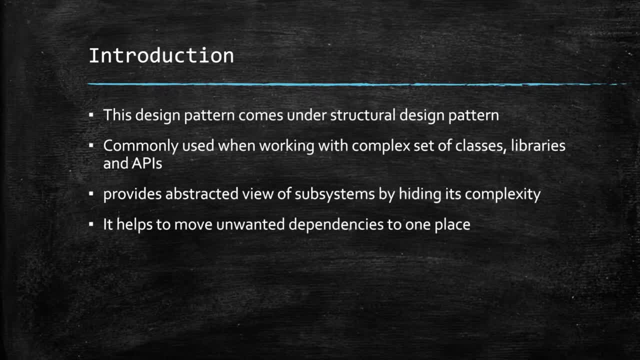 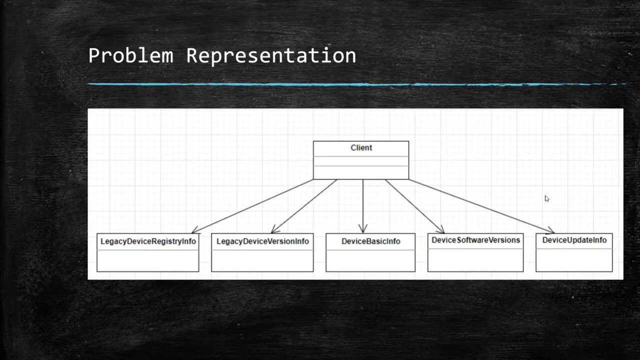 to provide simple interfaces as an entry point to access complex systems. now let's look at the examples, actually, which we are gonna take. first we will see the presentation of the problem and then we will go to the actual implementation. okay, so this is the problem: representation for our 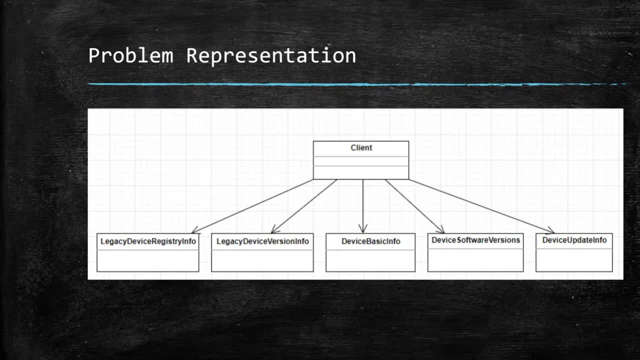 2ds demo. so actually the, the project actually which i have created for 2ds demo, is a device management system. so what it does: it collects the information from the device. device will be like laptop or computer. so what it does from the system, it gathers all the required information. like what? 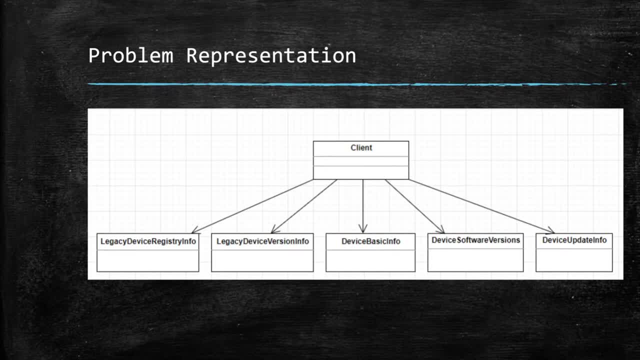 is installed, what is the version of the software or or the serial number of the device- ram capacity, hard disk space- then it also gathers information related to legacy devices. see, i'm using some external devices which are connected to my laptop to carry out certain operations, so i'm calling. 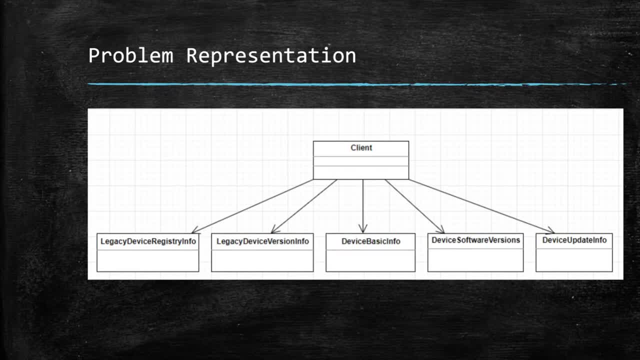 those devices as a legacy devices. so those device will also have some information which will be stored with my laptop, or that information may be with the legacy devices only and my laptop can communicate with them to gather that information. so this kind of functionality this uh project is having, so as of now, in a normal scenario what we are doing, is from our client. 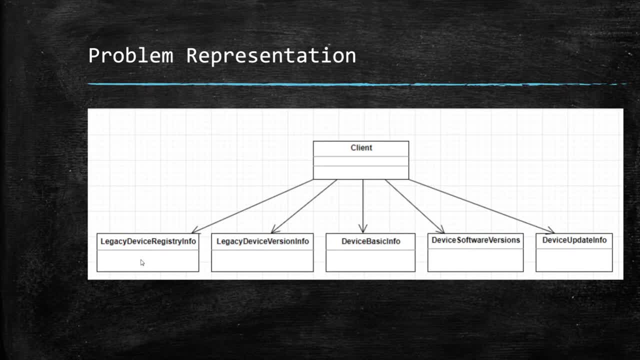 class only. we are providing him, uh, all the methods to gather this information, like legacy device registration for legacy device version info, so on. so right now the client is calling all these methods directly. so he has to instantiate all the classes and then call the respective method, gather the information and create an object, or i will say device info object, from that and then 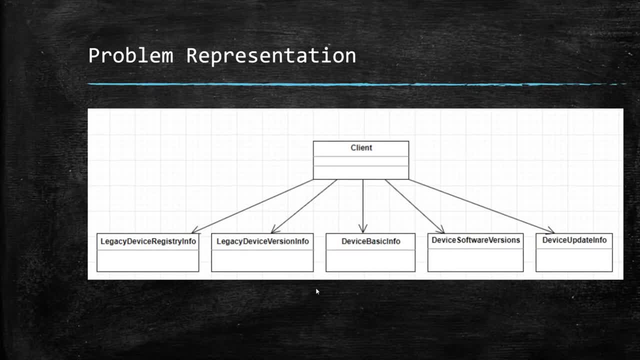 the database. so now, if we are creating all the instances of these classes in our client class, so somehow we are, we are tightly coupling all these subclasses with our client and it will become complicated because having these many instances that calling each other in case if we forgot to do something or call one method, so that then we will be in problem and in case if 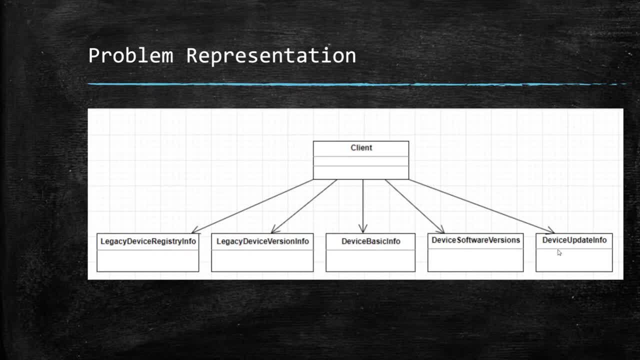 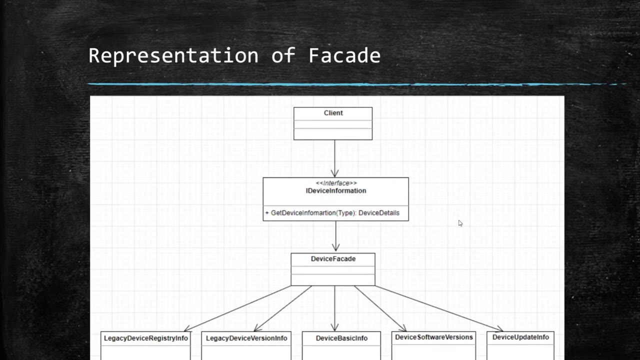 in future. uh, there are any changes to any of the method or any of the class, so that time we will need to touch our client as well, so which is not ideal. so to solve this, we are going to use facade design pattern, and how it helps. let's go to the next slide. yeah, so this is the solution actually. 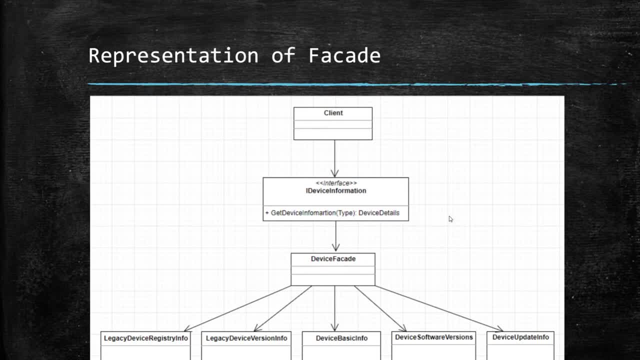 which we can design to handle this situation in more, better way. so what we have done is now we have introduced the facade class- we call it as a device side, and then we have created one interface as well. so we want to make our system a loosely coupled apart. so what we have done, we have 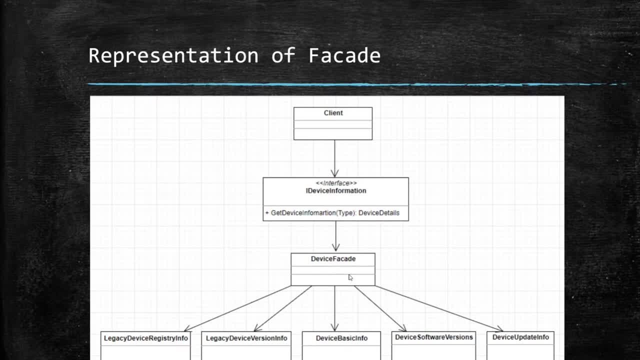 an interface as well, which client will be using. and then we have created one class, that is device facade class, and this device facade cloud actually will be communicating with all the subsystems, like legacy device registry info, legacy device version info. so with all these classes, this facade cloud will class will communicate, so it will have the responsibility of instantiating and 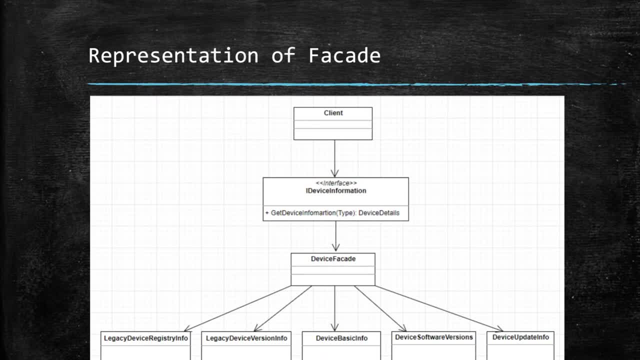 then calling the different, different methods gathering that information, and then what are the responses uh receiving? so collect all that response and pass it to the client. so we are unsure how to manage the task, this entire task of creating instances and gathering information from client to the device side, and in case if in future some other client comes requesting the same. 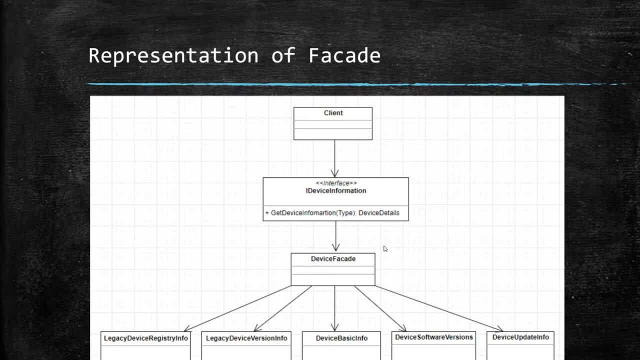 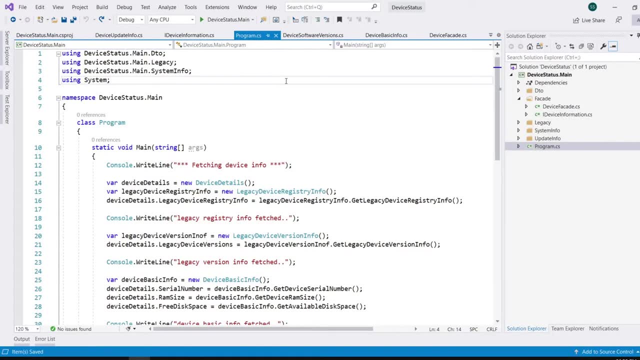 operation. he can directly call the device officer class. so let's now go to the visual studio and look at the actual implementation of this. okay, so this is the sample program i have created for demonstrating facade design pattern. uh, this project, actually, this is for managing the device. 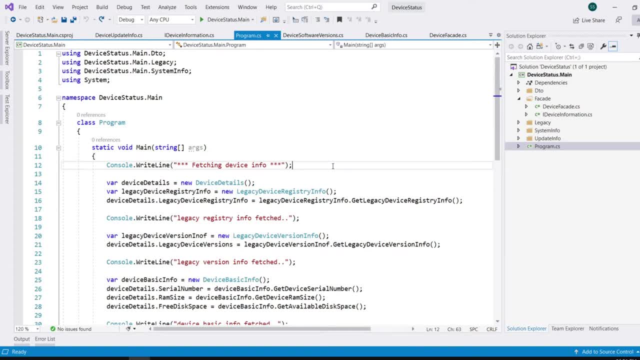 information. so for device status information. so when we say to create theimizi just, you can use these types of environment, you can use in other device sense and …. and then we'll talk about how to four say device status information. so what it does from registry or from system info it fetches. 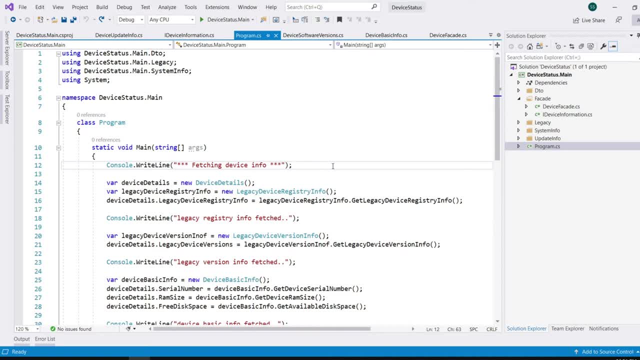 the basic information related to devices like ram size, what is the serial number, then what are the different softwares which are installed and what are the different software versions, as well as update history. and then there are two more scenarios where we fetch information related to legacy devices, and when we say legacy devices, those are the devices, old devices, which we connect. 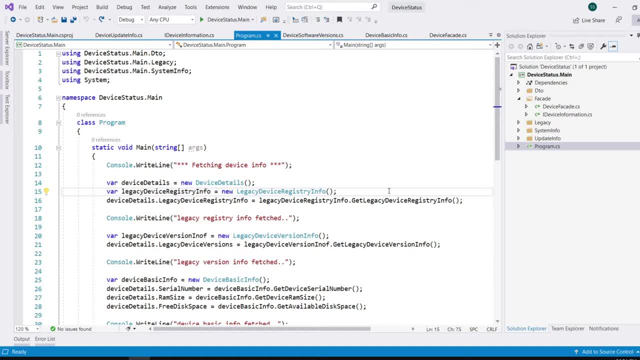 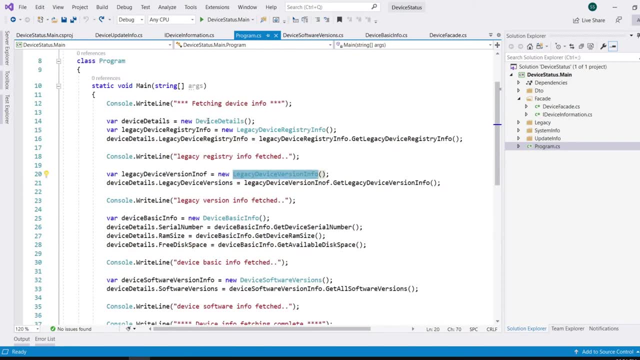 to our laptop to carry out certain operations. so when we connect those devices, uh, its information will be collected by system and that information will be fetching where these classes. so as of now you can see this is our client class programcs, because this will be actually display our 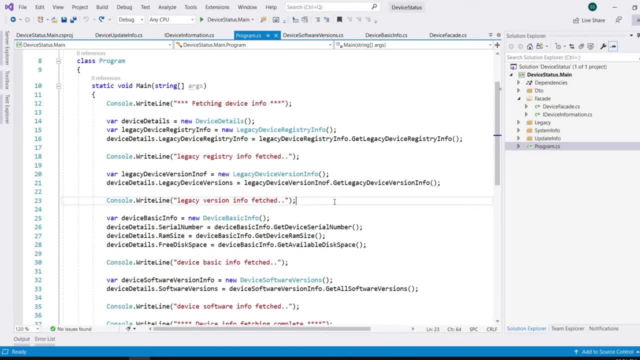 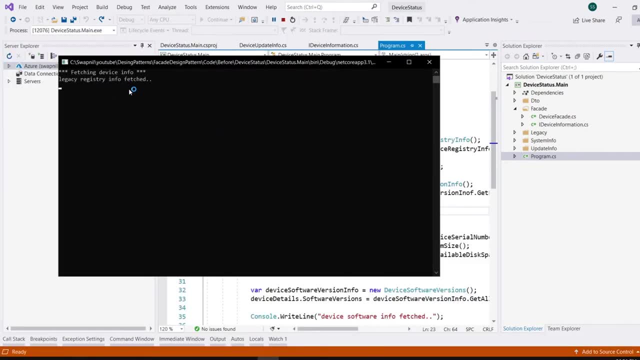 fetching out this information. so, as of now, let me run this program and show you the output. yeah, so you can see it has started fetching out the information and the logs related to fetching are are outputted on the console and you can see the fetching operation is complete. so now for fetching all this information. what we 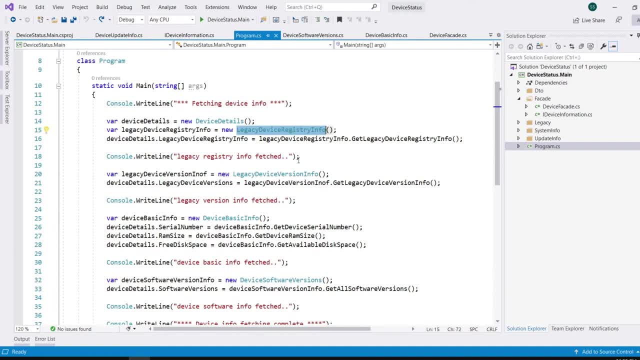 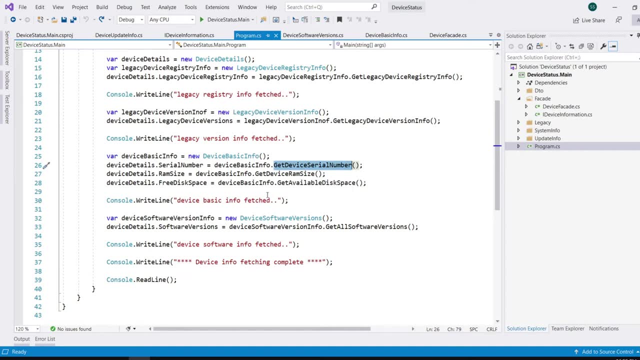 needed to do is we created instances of all these classes in our client application or in our client class, and then we are calling the respective methods and fetching all that information, then collecting that all information in one object, and then we pass it to database. so, as you can see, 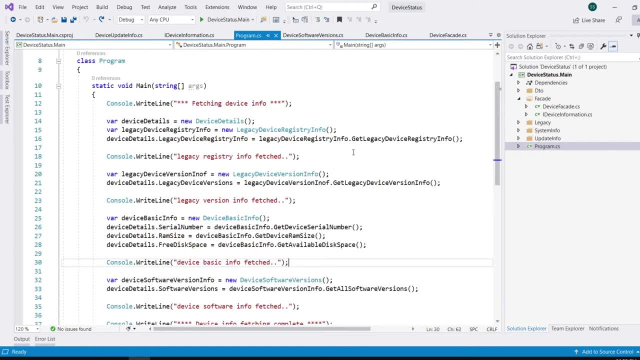 our client class is now tightly coupled to this. all these classes. we are instantiating it here, so this is the extra headache which client is having. so this is not a good practice. and in order to solve this kind of issues or problem, because in case in future, if something changes or we change this method, name or 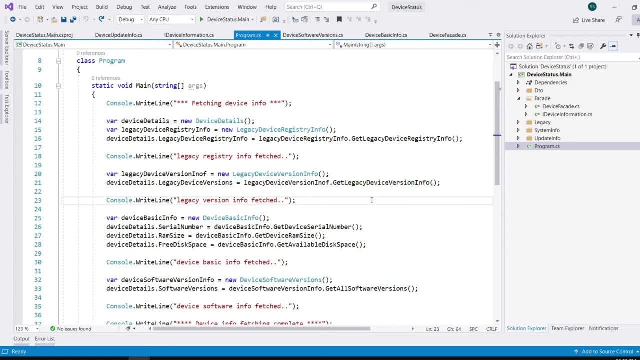 if this method starts accepting certain argument or something, so in case of signature changes, so in those cases we will need to touch the client code as well, because that time this method won't be available, so we will need to make changes in client code as well. so to avoid this kind of scenario. facade design. 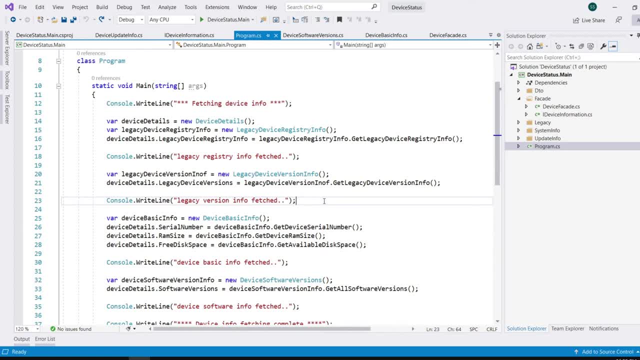 pattern actually comes out of our client class and then we are going to use this handy. so how to implement it? actually I have already done the code changes for same and we'll just show it to you directly. so to handle this scenario, what I have done, I have created one interface. this is I device information. it has only 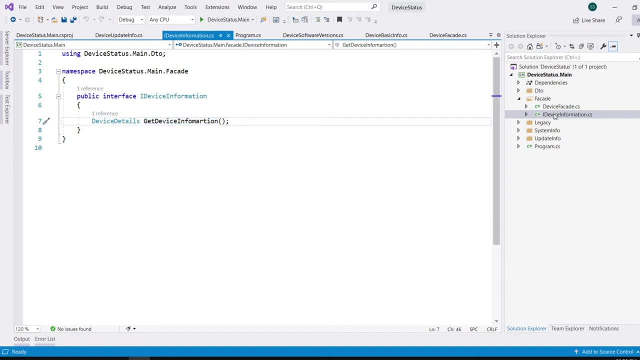 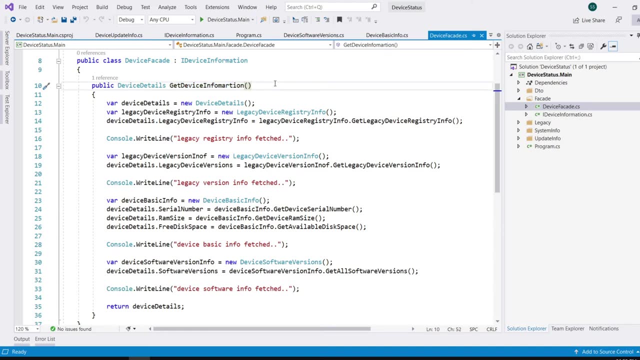 one method declaration, that is, get device information, and this particular interface is implemented by this device facade class. now, in the implementation of this gate device information method, we have done all the things which are required for fetching the information for different, different devices, or was a different system information? so whatever we were doing so 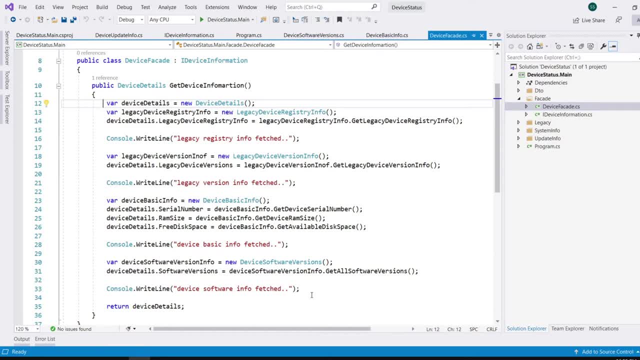 far in client class. we have moved that to this device facade class. so this class will now hold the responsibility of calling all these classes and gather all the information and just send the final output to our client code, or can't, client class. so now, once we have done this changes. so now to consume that. 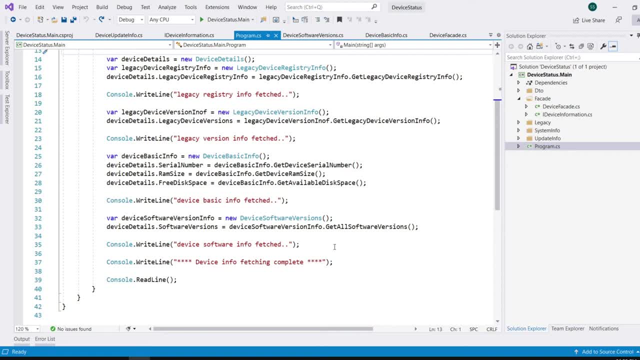 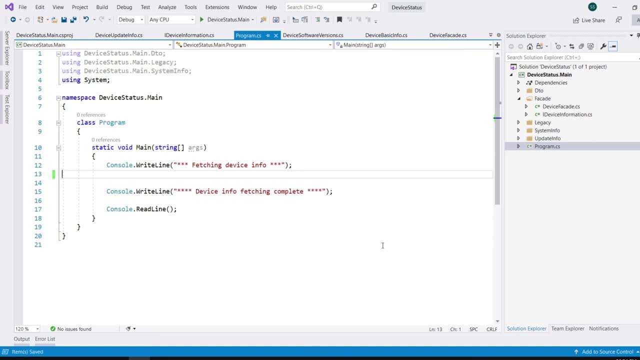 we only need to know code. so I will do those changes right away. so let me just remove this much code now because it is not required anymore. yeah, so now we just need to instantiate device facade- so yeah, so instantiated, and call the respective method- you, we have logged it to access the educational resource and.